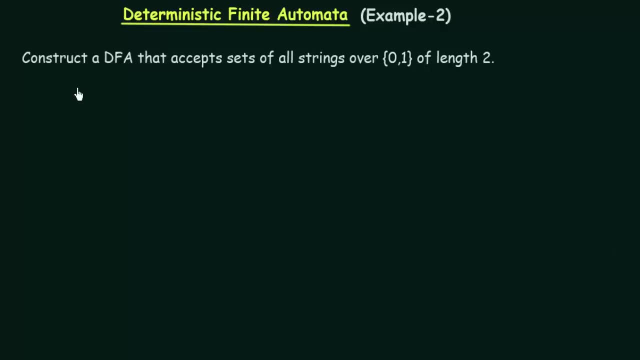 But before that, let's see what are our alphabets. Our alphabet set here is 0 and 1.. It's already mentioned here 0,1.. And what will be the set of strings in our language? Our alphabet set is 0,1.. 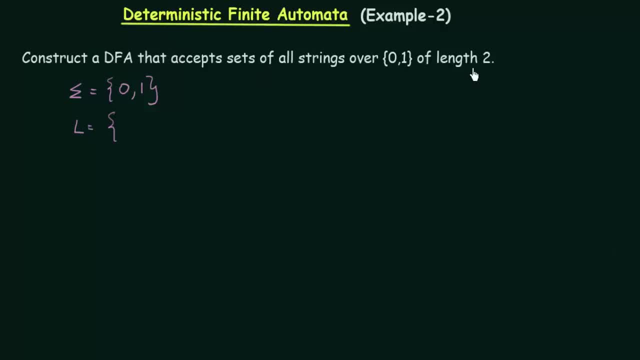 And all the sets, sets of strings over 0,1 of length 2.. So what are the set of all possible strings of length 2 over 0,1?? They are 0,0,, 0,1,, 1,0 and 1,1.. 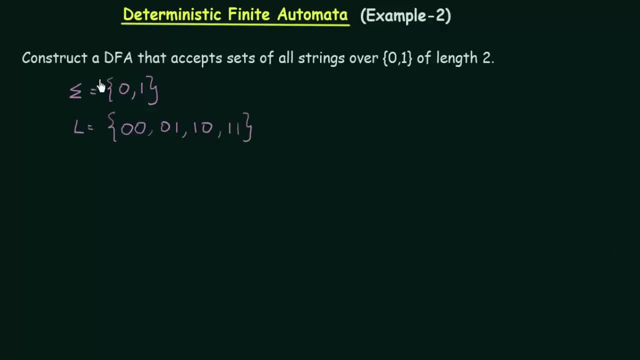 Okay, so we should construct a DFA that accepts 0,0,, 0,1,, 1,0 and 1,1.. These are the only 4 inputs that should be accepted by the DFA that we are going to construct. 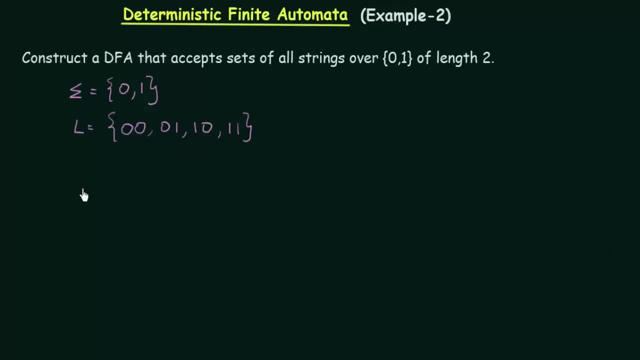 And it should reject all alphabets And it should reject all other strings. So let's see how we can do this. Okay, so, to start off, we always need to start with the initial state, or the starting state, And let me call it A. 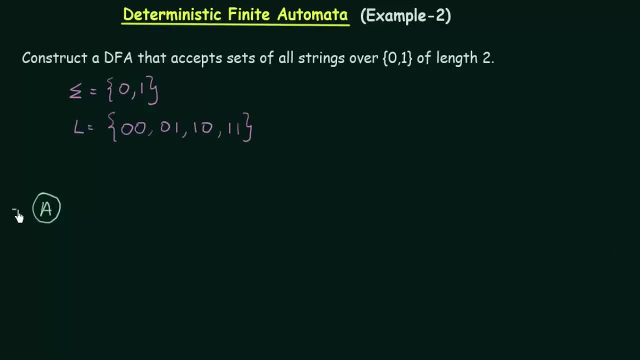 A is my initial state or starting state, And how do I indicate that it is initial state or starting state By this arrow? This arrow, which comes from nowhere, pointing to state A, indicates that A is the initial state or starting state. Okay, Now we have to mention what happens if A gets the input 0 or 1.. 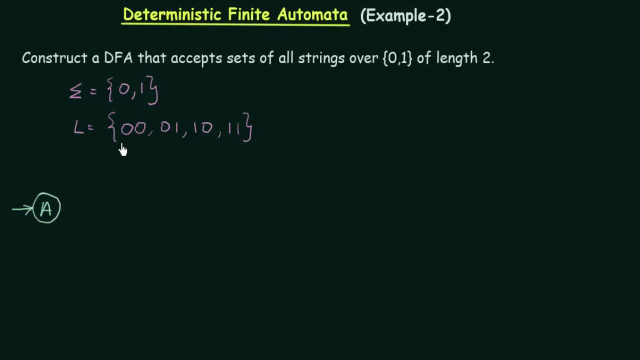 So here it does not matter what is the starting string. It could either be 0 or it could either be 1.. The only condition is that it should be of length 2.. So whether I get input 0 or 1,, I send this A to the next state, which I will call B. 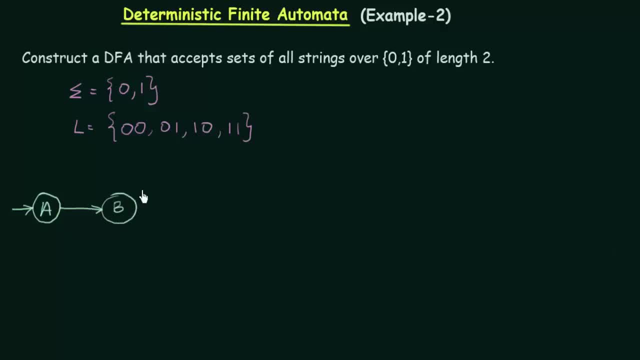 Okay, If A gets the input 0 or 1, it goes to the next state called state B. Okay, So at this point, when I reach state B, what is the length of my string? The length of my string is 1.. 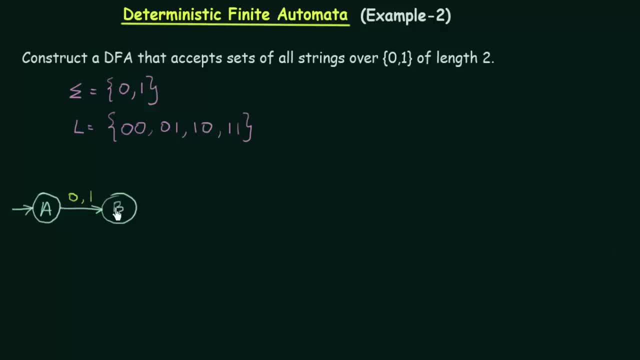 Why? Because I was in state A and I just came to the next state- First state, second state- So I just came here, So I got input either 0 or 1.. So the length of my string is 1 at this point in B. 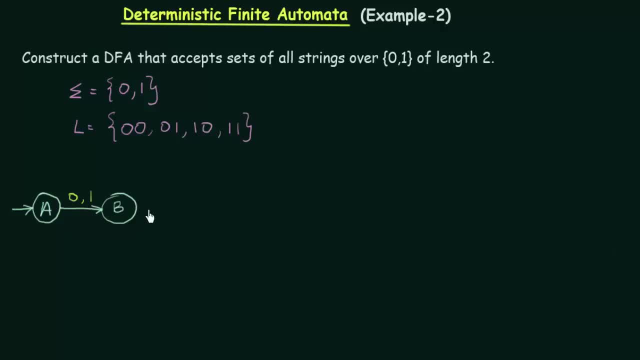 Okay. So now we have to mention what happens if I get either input 0 or 1 in state B. Again, the order does not matter, So I send this B to the next state, which I will call state C, Whether I get input 0 or 1.. 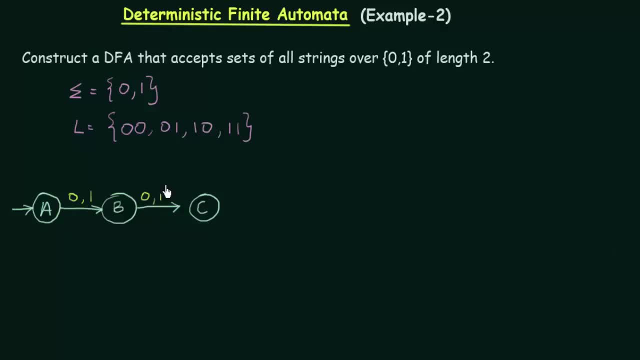 0 or 1 in state B, I send it to the next state, which I call state C. And at this point, when I reach state C, what is the length of my string Here? when I came from A to B, the length of my string was 1.. 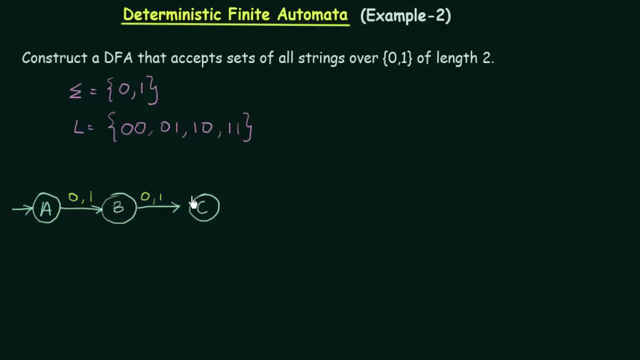 And when I go from B to C, what is the length of my string? It is 2, because I have already got 2 inputs. So, and the DFA that we construct should accept all strings of length 2.. So if it reaches here, the length is 2.. 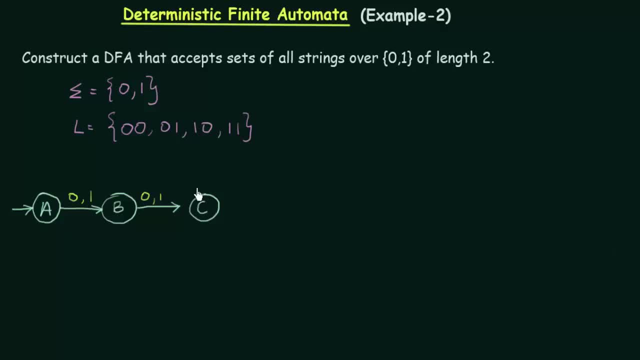 That means that should be the accepting state or the final state. So I have to put a double circle around this C, indicating that this is the final state, Right? So here, at this point, the length of my string is 2. And that is the final state or the accepting state. 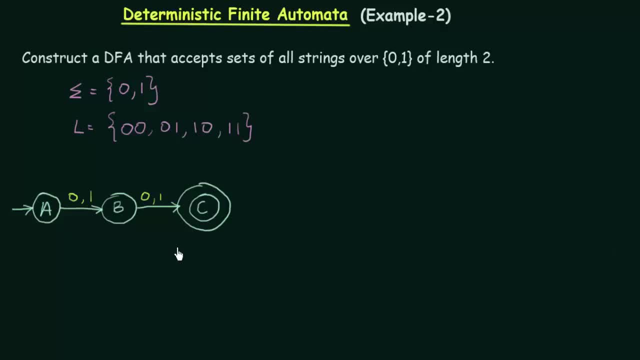 Well and fine, Okay, But is this DFA complete? No, it is not complete. Why is it not complete? Because I have already mentioned that. I have already mentioned what happens if I get 0 or 1 input for A. I have also mentioned the same thing for B. 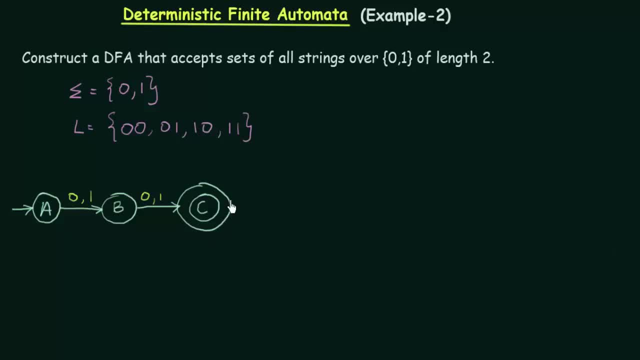 But what about C? C is not complete. I did not mention what happens if I get an input again in C. So what happens? Whether I get input 0 or 1 in state C, I will send it to another state, which I will call state D. 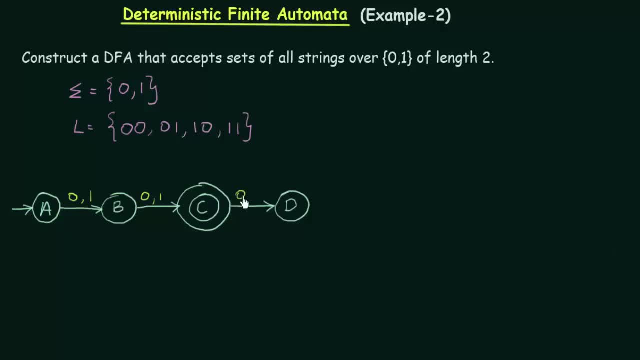 Okay, Whether I get input 0 or 1, I send it to state D And in this state D, this also is not complete, because I did not mention what will happen to state D, Whether it gets 0 or 1.. 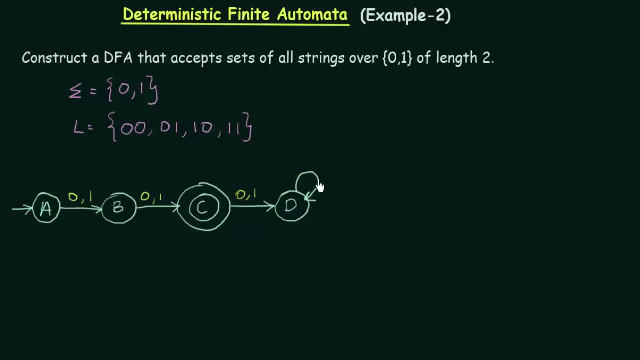 So I give a self-loop to state D, saying that whether I get input 0 or 1, it stays in state D itself. Okay, It stays in state D itself. Now, what is the meaning of this? So, at this point, 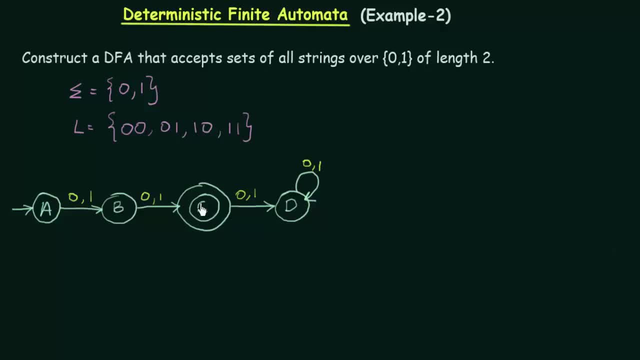 when I reach state C, I already got the length of my string as 2.. Now if I get another input, the length of my string becomes 3. And that should not be accepted. So it goes to this state D. 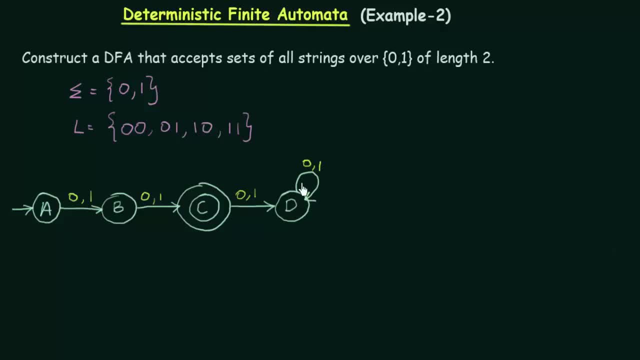 And after reaching state D, whatever input you get, it stays in state D And from state D there is no possibility of coming back to this state C, which is the final state. So if anything goes out of this state C, 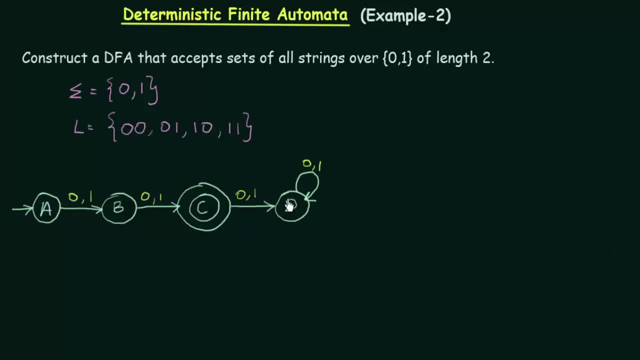 it stays here And it is trapped here, Not being able to reach the final state anymore. So any string of length more than 2, it goes to state D And it is trapped here And it will never be accepted. So this state D here is known as the. 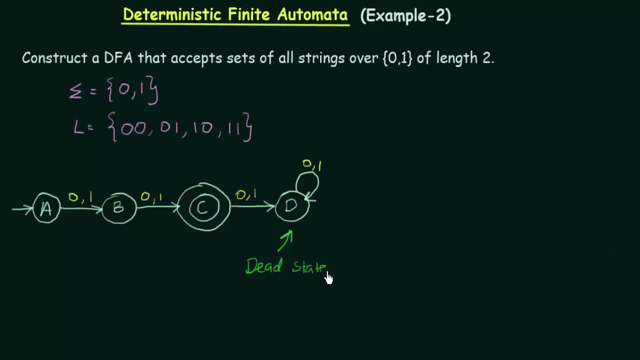 dead state. It is known as dead state, Or it is also known as trapped state. Okay, Now my DFA is complete, Because I have mentioned for every state what happens when I get a particular input, Either 0 or 1.. 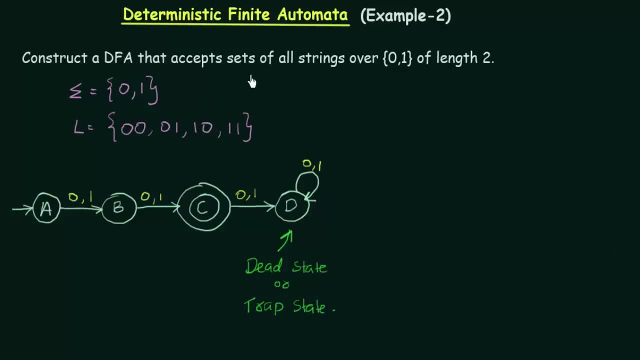 Now I have successfully designed the DFA that accepts sets of all strings over 0,1 of length 2.. Alright, I hope that was clear. Now let us take a few examples and check if this is working. So here we will take a few examples. 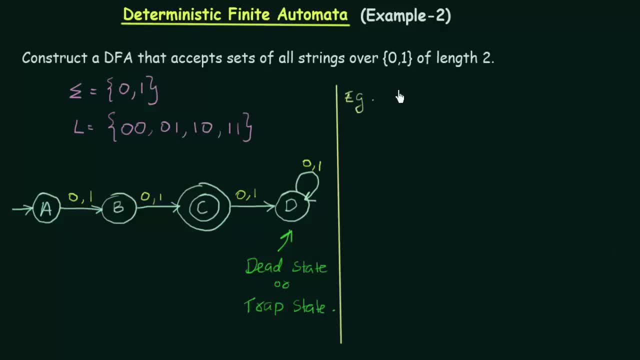 So for my first example, let me check the string 00.. So 00 should be accepted. actually, 00 is present here And it is of length 2. So it should be accepted. So we always have to start with our. 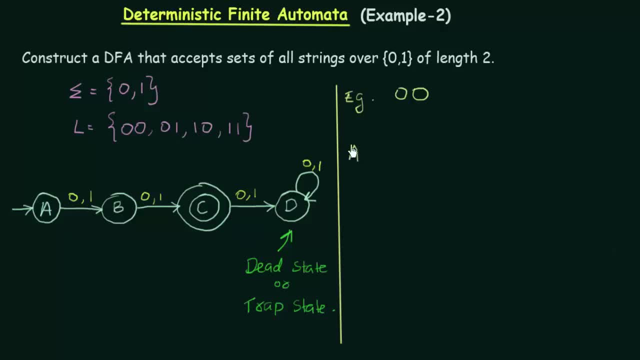 starting state, which is state A. This is my state A. I am starting from here And the first input is 0. So I get input 0 in state A. And what happens When A gets the input 0, it goes to state B. 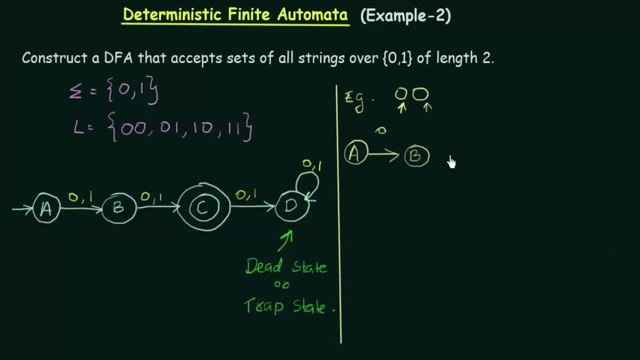 And what is the next input? The next input is again 0.. Right, 0.. I am in state B right now and I get input 0. So in state B, if I get input 0, where does it go? 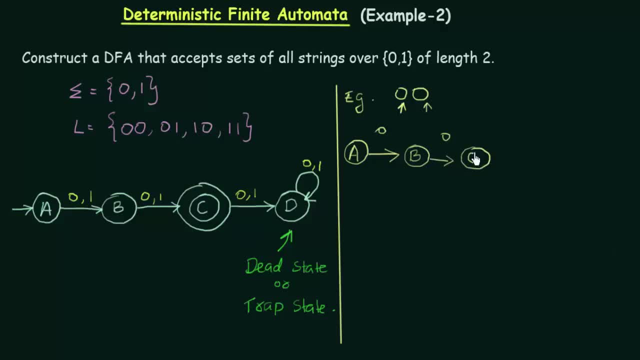 It goes to state C, It goes to state C, And now I have reached the end of the string, And at the end of the string I am in state C. And is state C the final state? Yes, it has a double circle, which means 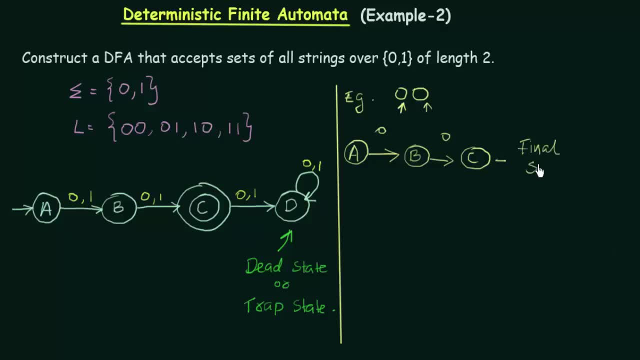 it is the final state. Now, since state C is the final state, this is accepted. Whenever a string reaches the final state, it shows that it is accepted. So 0, 0 is accepted. Now let's check another one. 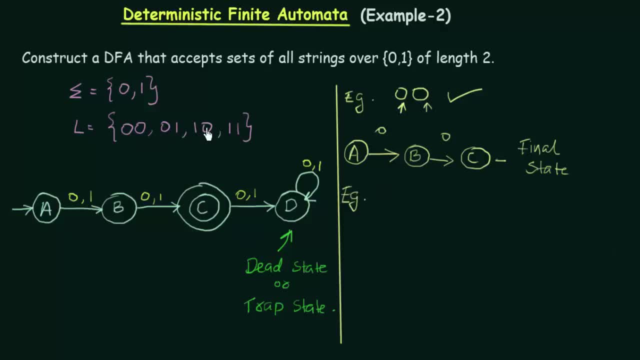 Let's check for 0: 0.. Let's check for 1: 0, now 1: 0.. Again, I start from my initial state A And the first input is 1.. So I am getting input 1.. 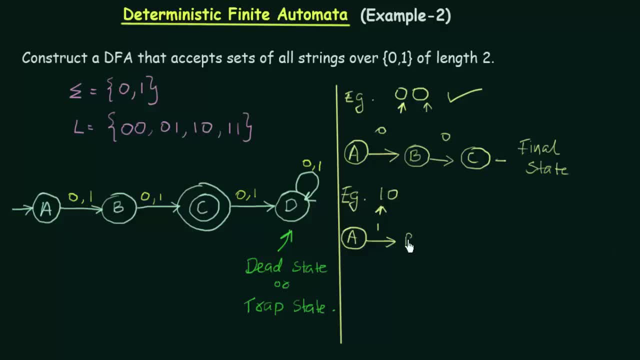 What happens to state A? It goes to state B. Right, And now the next input is 0.. So what happens? I am in state B and I get input 0.. I am in state B and I get input 0.. 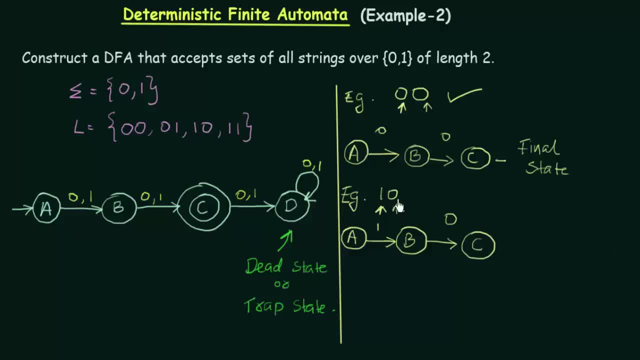 It goes to state C. It goes to state C And I have reached the end of the string. And at the end of the string, where am I? I am in state C. Is C the final state? Obviously it is. 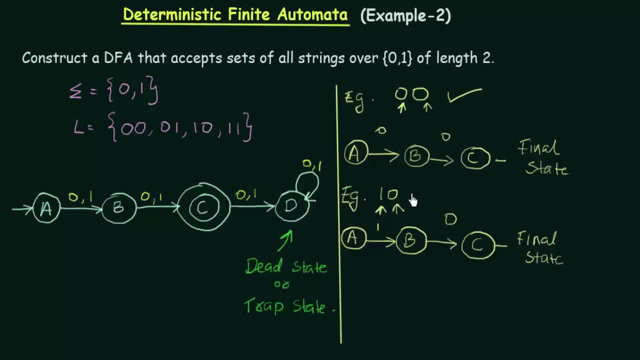 It is the final state, So this is also accepted. Why? Because it reached the final state. So far, so good. Now let's check for a longer string, Which is 0 0 1.. Let's see if this will be accepted or not. 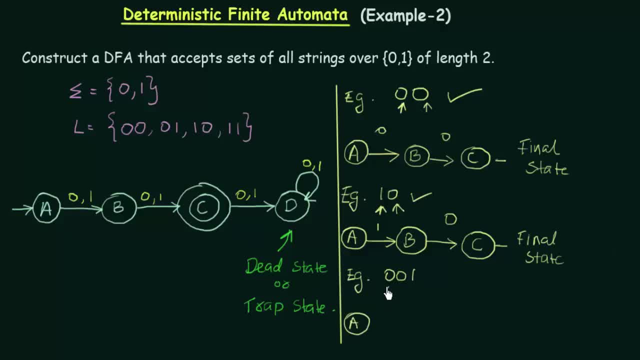 Again, I start from my initial state. A First input is 0.. So I get 0.. What happens In A? if I get 0, it goes to B, It goes to B, And now I am in B. 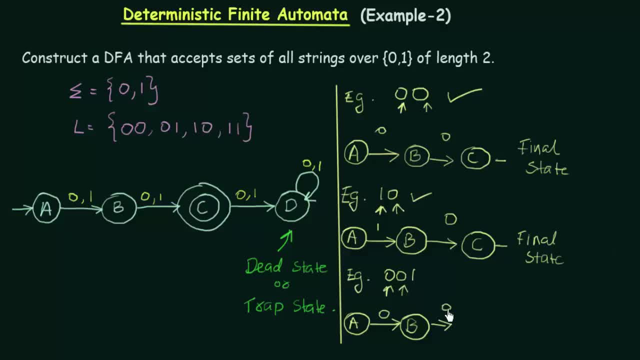 And the next input I get is again 0. So when I get the input 0 in B, it goes to state C, Right, And again I have one more input here, which is 1.. So I am in state C.